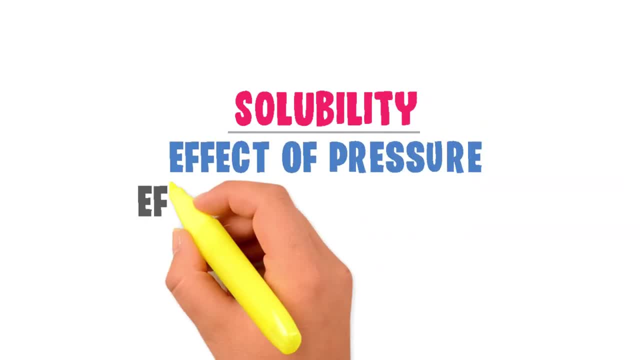 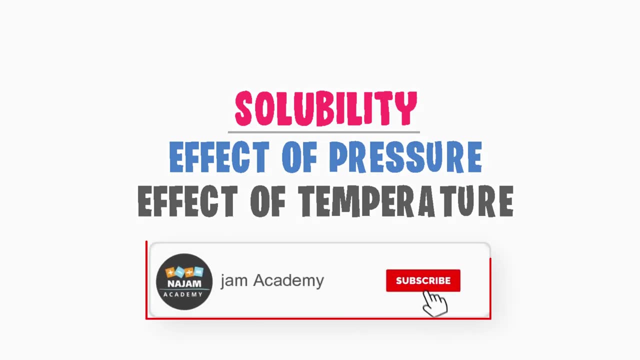 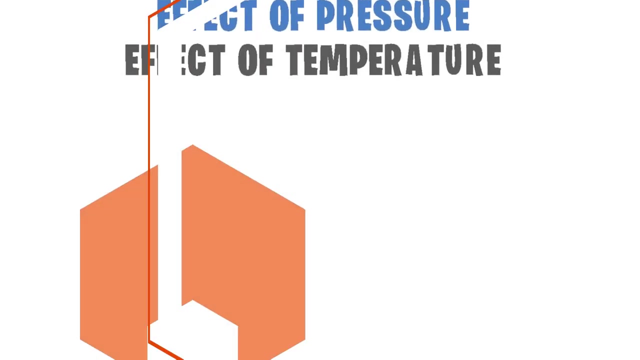 What is solubility? effect of temperature on solubility and effect of pressure on solubility. Before starting the lecture, click on the subscribe button and get access to our 100 of conceptual lectures for free Now. what is solubility? 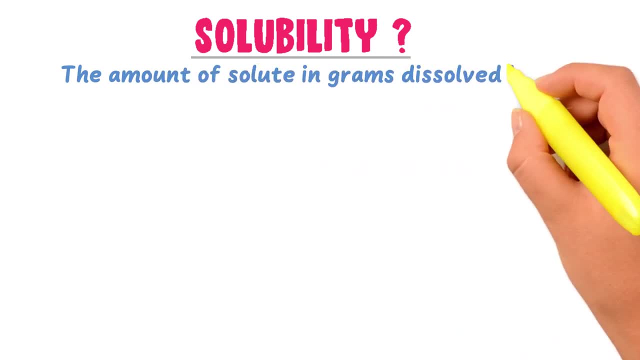 Well, the amount of solute in grams dissolved and 100 grams of the solvent to prepare a saturated solution at a given temperature is known as a solubility. For example, consider 100 grams water and this beaker at 30 degree centigrade or at room temperature. 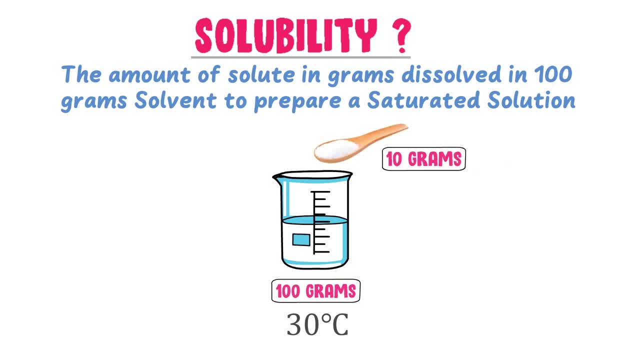 Firstly, I add 10 grams sugar and 100 grams water. It is easy, It easily dissolves in the water. Secondly, I again add 10 grams sugar and 100 grams water, But this time some sugar dissolved in the water and some sugar settled down at the bottom. 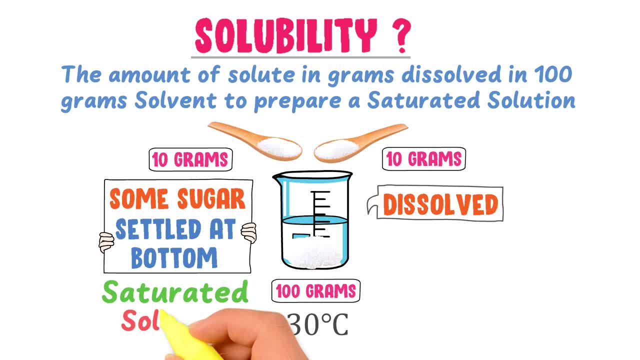 This means we have prepared a saturated solution of sugar and water at 30 degree centigrade. Now listen carefully. I dissolved 20 grams sugar and 100 grams water, Such that I got saturated solution. Saturated solution means that 100 grams water can only dissolve 20 grams sugar at 30 degree centigrade. 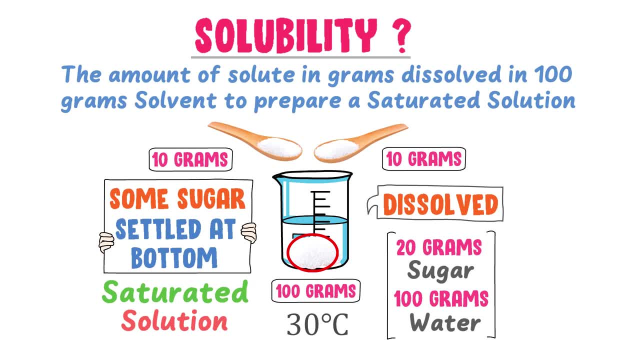 The extra sugar would settle down at the bottom. Thus we say that the solubility of sugar is 20 grams and 100 grams water at 30 degree centigrade. Let me repeat it: The solubility of sugar is 20 grams and 100 grams water at 30 degree centigrade. 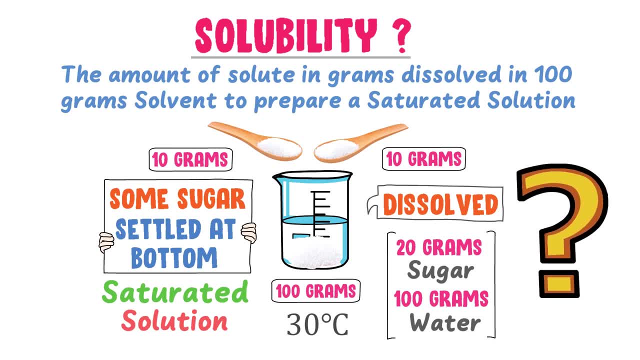 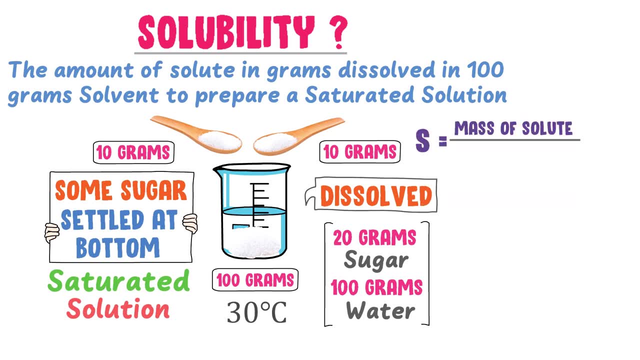 Now, how can we calculate the solubility of a solution? Well, the formula of solubility is equal to mass of the solute over mass of the solvent and 200.. Here, the mass of the solute, or sugar, is 20 grams that are dissolved and 100 grams solvent or water. 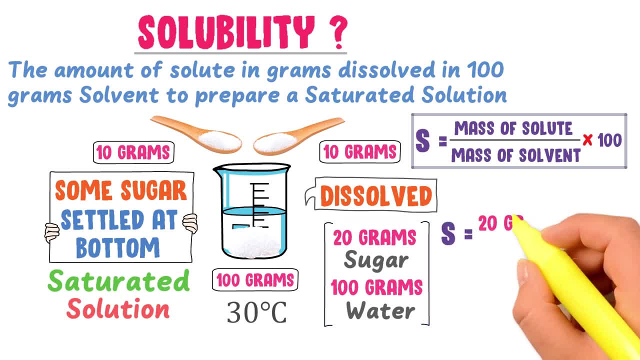 Hence we write: solubility is equal to 20 grams over 100 grams and 200.. Thus we get: solubility is equal to 20 percent. It means that the solubility of sugar is 20 percent and 100 grams water. 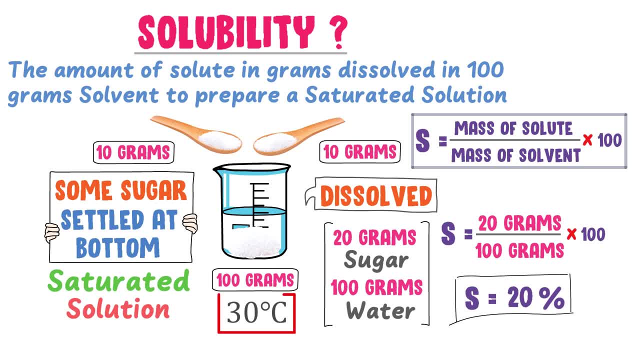 At 30 degree centigrade. Here, if we increase the temperature of water, solubility of sugar will be increased. Thus, remember that solubility means how many grams of solute is dissolved and 100 grams of solvent at a particular temperature. 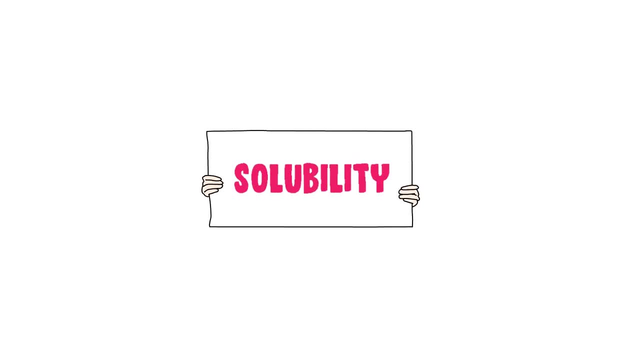 Finally, let me teach you that solubility depends upon three factors: Nature of solute and solvent, Pressure And temperature. For instance, the solubility of salt and water at 30 degree centigrade would be higher than the solubility of sugar. 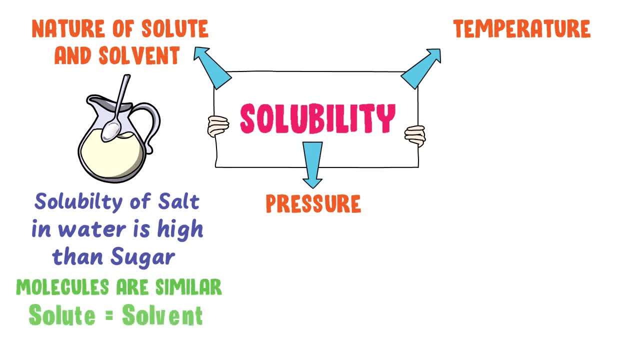 It is because when the molecules of solute are similar in structure and properties to the molecules of solvent, solubility is usually high. Secondly, if the solute and solvent are gases, solubility is affected by them. For instance, in carbonated drinks, carbon dioxide is dissolved in water at high pressure. 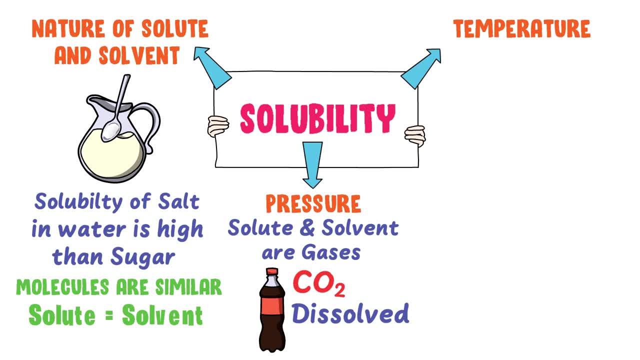 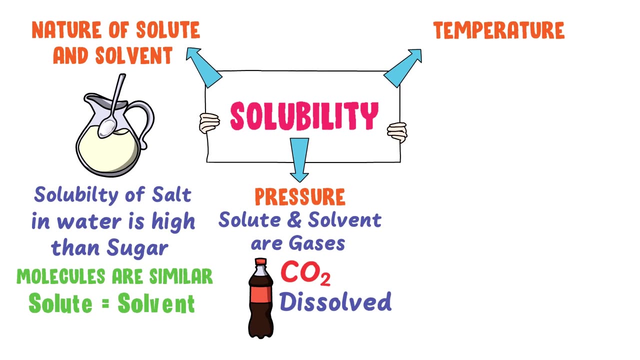 Once you open the bottle, pressure decreases and carbon dioxide gas evaporate. As a result, solubility decreases. To learn the effect of temperature on solubility, you must learn three chemical reactions: Exothermic reaction, Endothermic reaction. 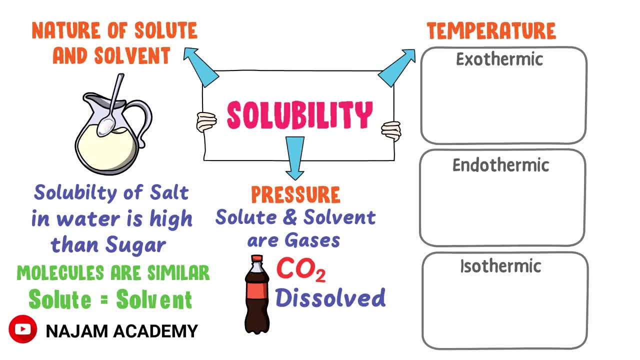 For example, when you add calcium hydroxide to the water, heat is released and the surrounding. This is known as an exothermic reaction. Here, if we increase the temperature, solubility of calcium hydroxide and the water decreases. 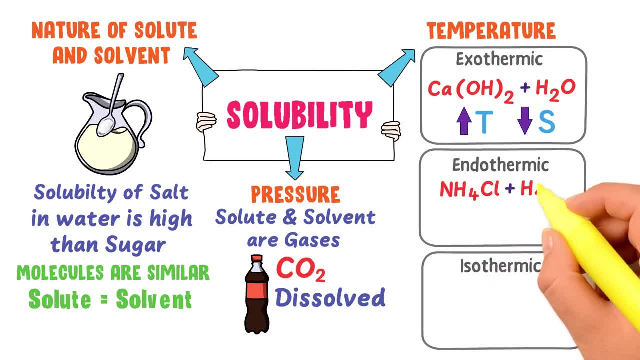 Secondly, when you add ammonium chloride to the water, heat is absorbed From the surrounding. So it is endothermic reaction Here. if we increase the temperature, solubility of ammonium chloride and water increases. Thirdly, when you add salt to the water, heat is neither absorbed nor released.